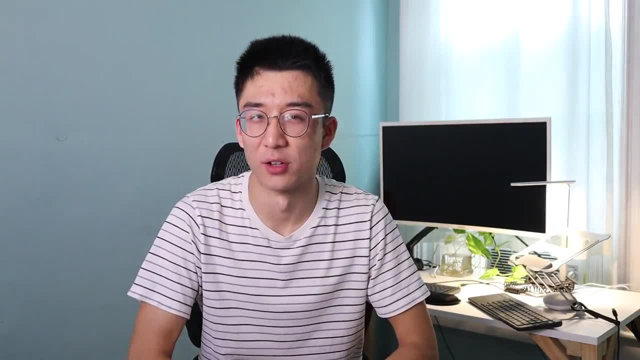 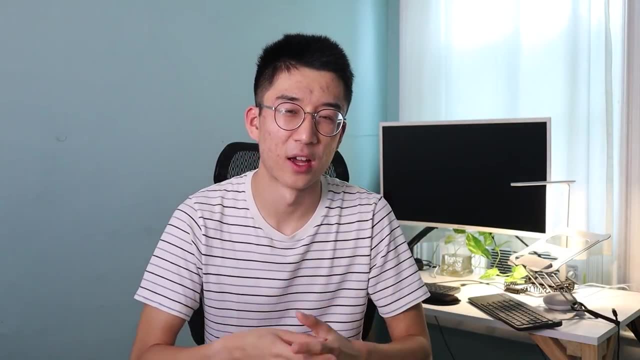 rising senior biomedical engineering student at Brown University. And yeah, that's pretty much it. I think in the process of getting to this point I've had many thoughts of, oh, these are things that I wish I would have done. Maybe it would have been better if I had done this. 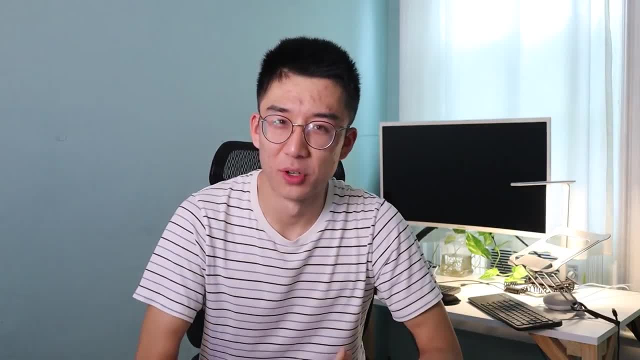 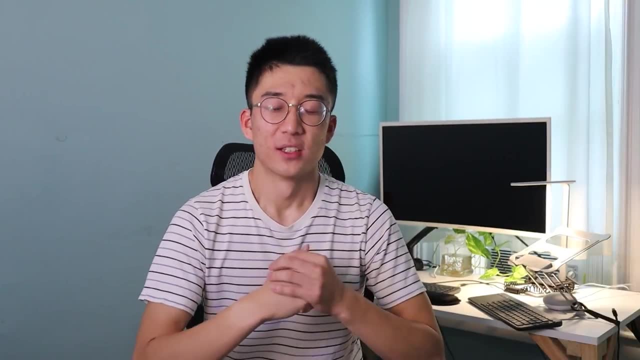 And so today we're going to be talking about that. Honestly, I'm like at the point where I just want to graduate but I still have a year left and I just feel like I don't want to take classes anymore. Anyway, let's go on to the first regret, And it is not understanding what the point. 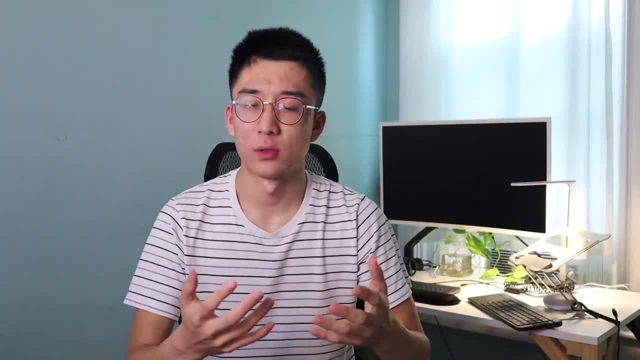 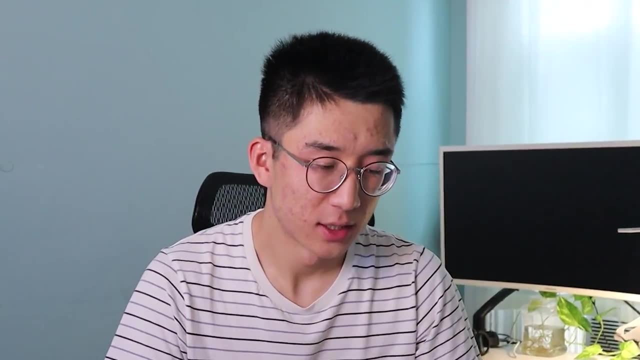 of my degree was going to be. And then you might be thinking, well, isn't that kind of dumb Like you're paying all this money for this biomedical engineering degree and you don't even know what it's going to be for. Well, kind of yeah. But my situation was: I came into Brown as a 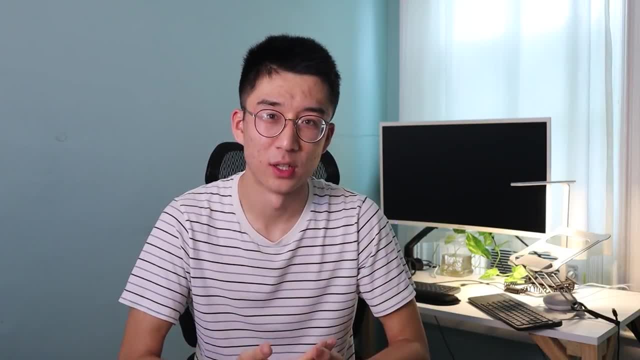 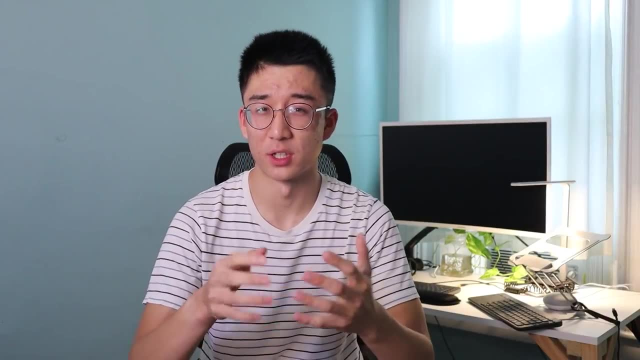 CLEME student, so I knew that I wanted to attend medical school. And then, as a freshman, I thought engineering was pretty cool, So that's why I decided to study engineering. But you know, in medical school I'm not really going to be using engineering much, And so my degree, like the 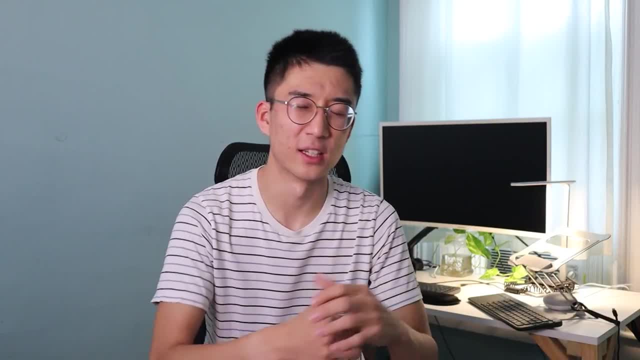 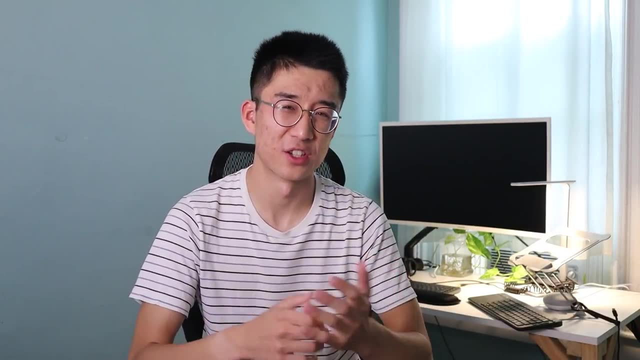 skills that I gained through my degree aren't going to directly transfer over to medical school. Pretty much most of the things that I've learned in my engineering classes I'll probably never touch again, And that's just kind of concerning, you know, given that I've invested so much time. 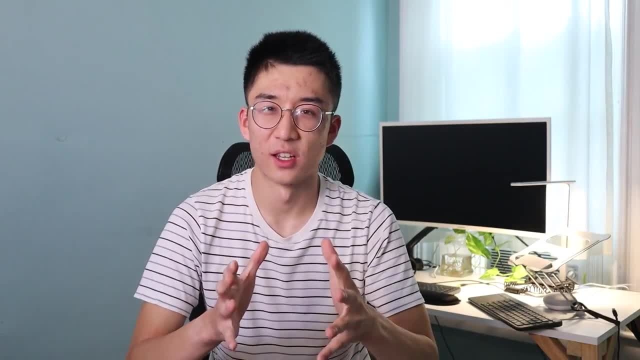 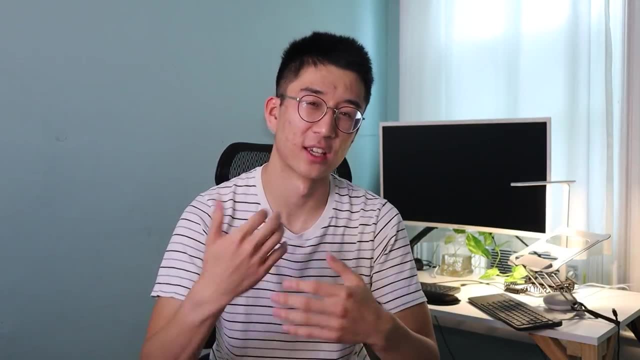 taking those classes and getting those grades. However, I don't want to say that everything I did was for waste, because I still think that going through the process- solving all those P-sets, taking all those classes- still may be the person I am today and has honed my problem-solving skills. so 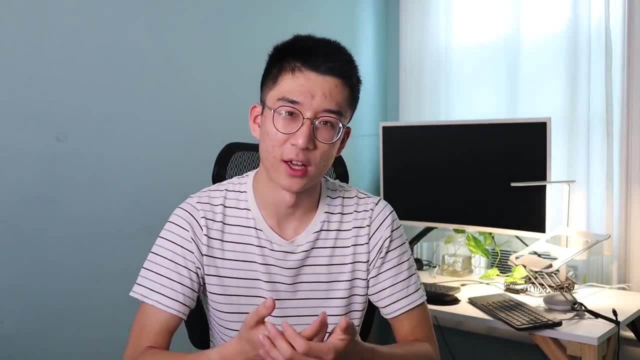 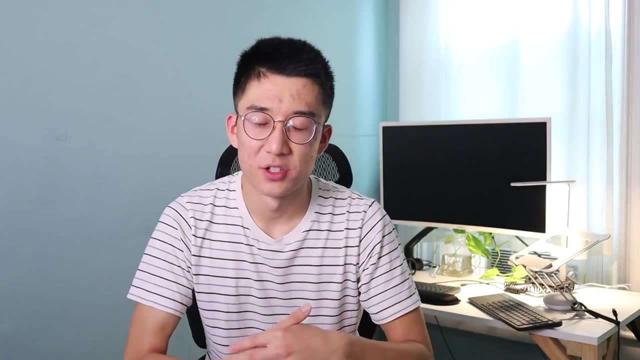 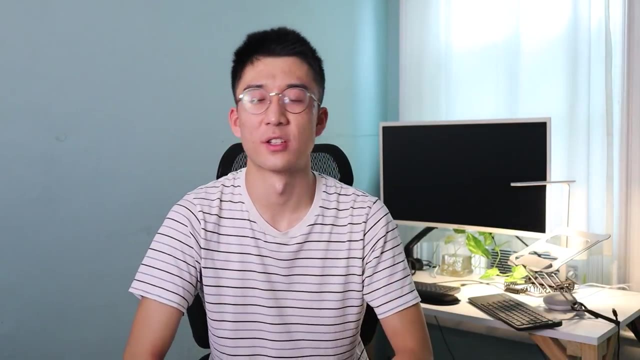 that I can think the way that I do, But I think that it would have been better if I had gained more clarity at the beginning of what I really expected to have. Biomedical engineering is such a time-consuming and intensive concentration, And there's so many other concentrations out there that are 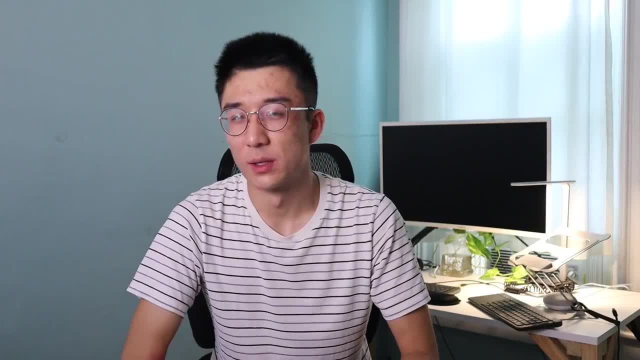 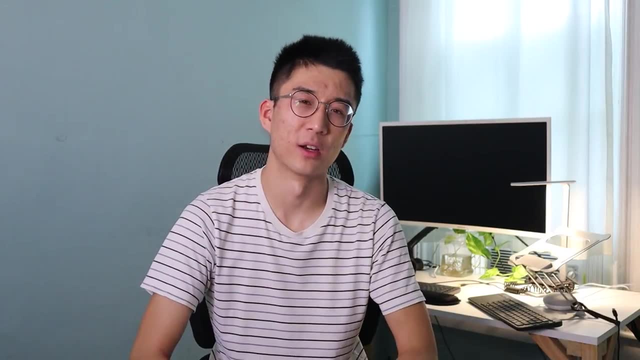 interesting and are useful. So maybe it would have been better if I had considered more of my options. But you know this is where I ended up And I do wish that I thought about it more as a freshman. So my second regret is kind of related to my first regret and it's not looking into. 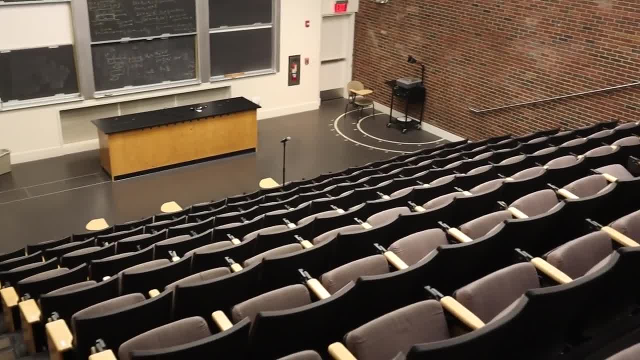 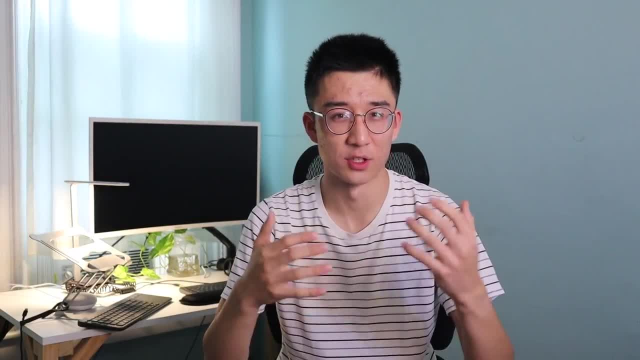 customization options for my concentration as a freshman, So I think this might be a little unique to Brown, but Brown offers students a lot of flexibility in terms of where they can go, what you want to study and how you want to structure your education, So I could have taken 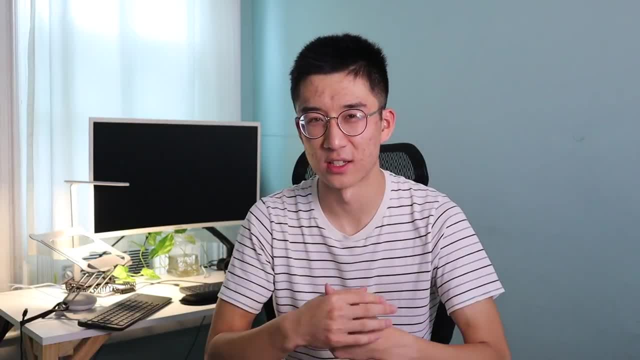 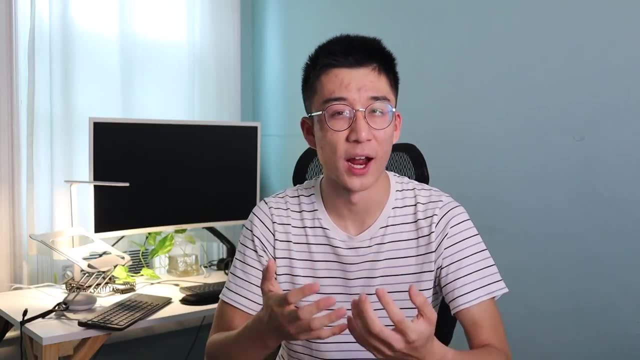 advantage of that and really changed up what courses I was going to take as a BME concentrator. But you know, I didn't really go into it and I kind of just decided to take the regular BME track And that kind of led to, you know, the situation I mentioned earlier, where a lot of the classes I'm 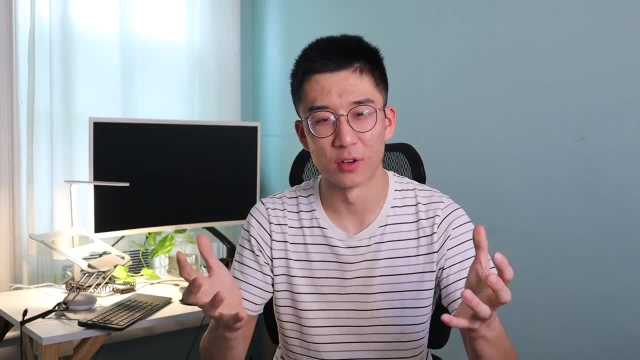 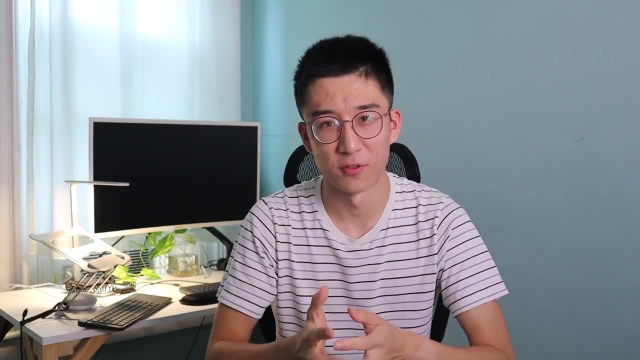 taking I'm probably never going to use anymore, or they just aren't very useful because they're so theoretical. So it would have been cool if I had gone in a different direction. For example, I know my friends who are studying biomedical engineering modified their degree to include more computer. 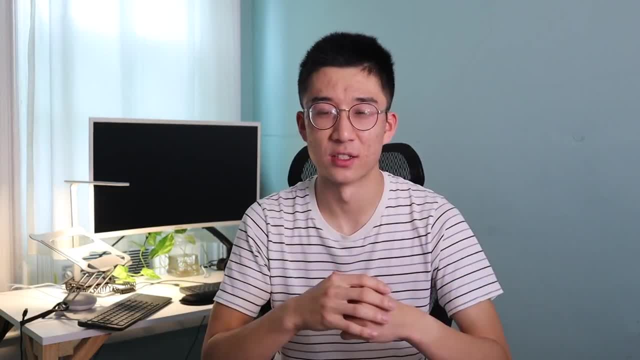 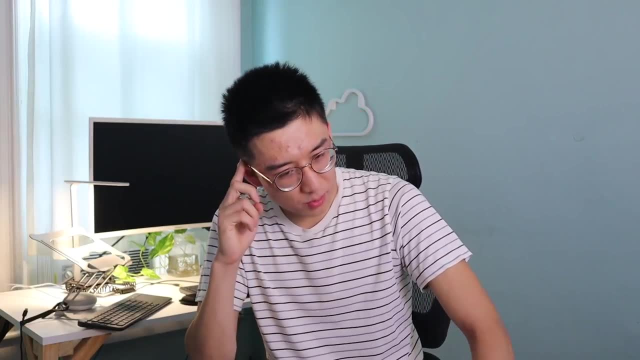 science classes instead of, like engineering classes such as thermodynamics, which, honestly, you're probably going to forget anyway after you take the class. So I think that would have been pretty cool in hindsight, even though at the moment I was just kind of naive and just decided. 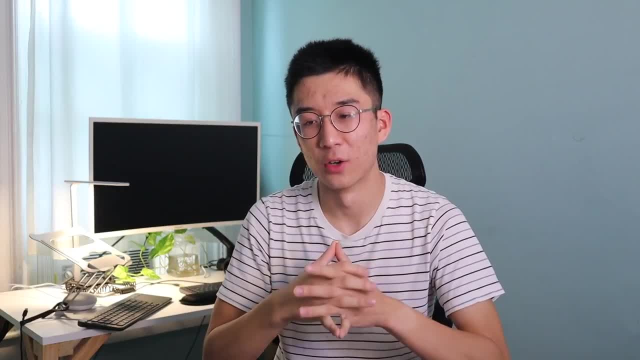 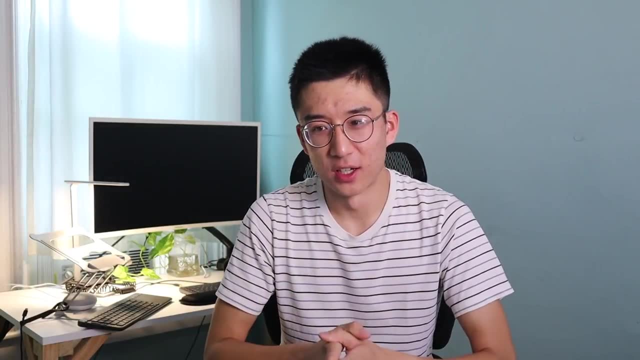 to go with the typical structure, But if I had known better when I was a freshman, I would have looked into more options, you know. So with the computer science example, I think that would have been really nice, since computer science is such an in-demand. 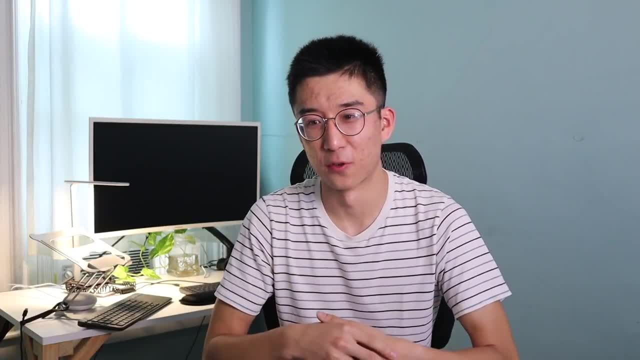 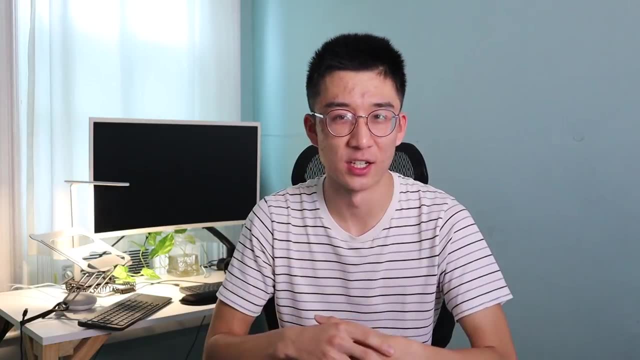 and hot field. right now. I'm actually doing software engineering for my summer internship, not biomedical engineering stuff, So that just shows you how important it is in today's day and age to be able to code, And so, yeah, if I structured my concentration to be more of that, then I 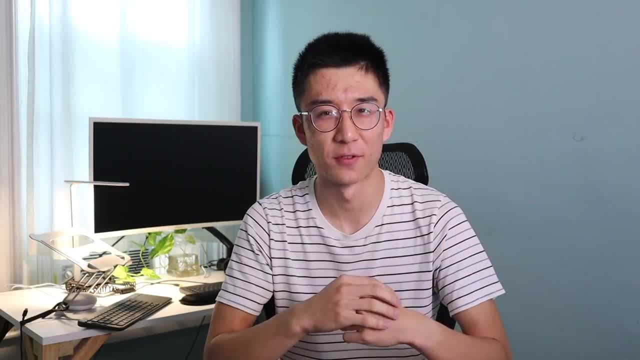 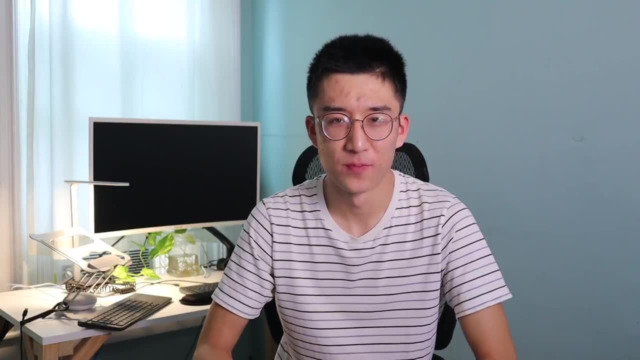 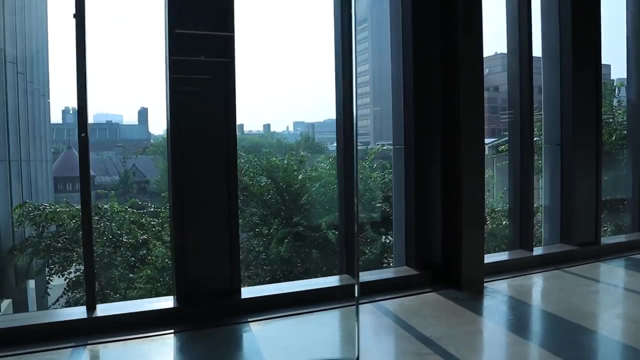 probably would have been more prepared to do more computer science-y stuff. You know, the more I talk about computer science the more I start to think of how I kind of regret my decisions in the past. But you know, it just comes with being jaded. Regret number three is neglecting office hours. 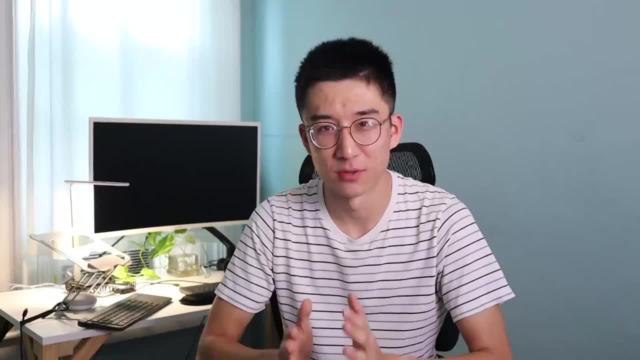 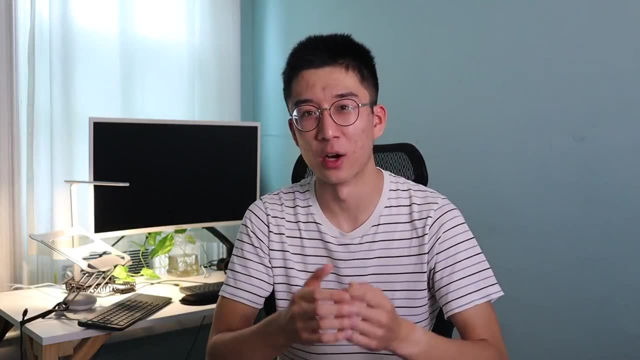 So this is kind of a big one for me. As a freshman I was really try-hard, I really wanted to prove myself in the classes And so whenever we had problem sets, I always wanted to finish them by myself. So I never asked for help. You know, I thought if I asked other people for help, 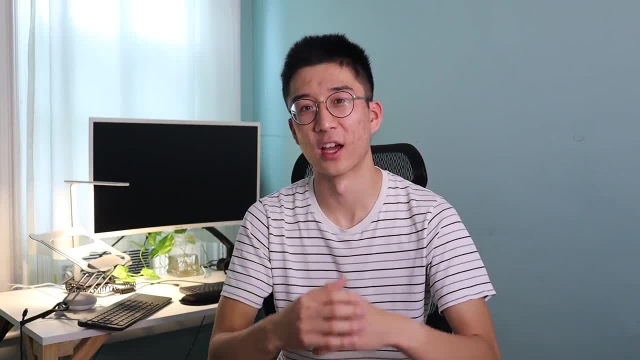 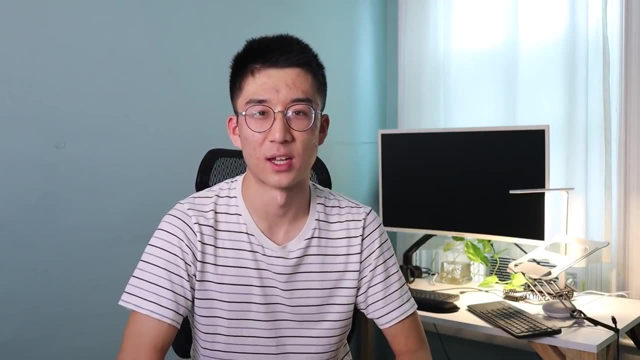 I would be giving up and that I wouldn't be prepared if I had internal help. In hindsight I was just so naive, because the nature of many of those engineering problems is that you have to have a certain intuition to be able to solve them. So you know. 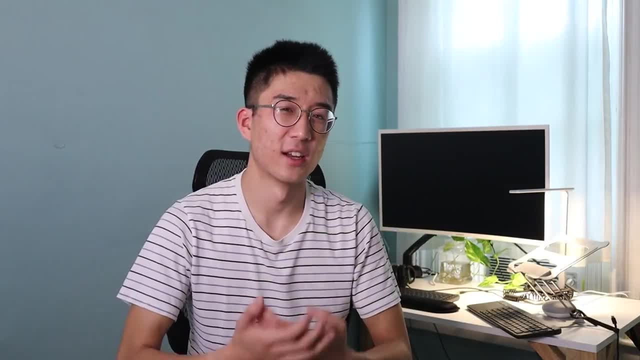 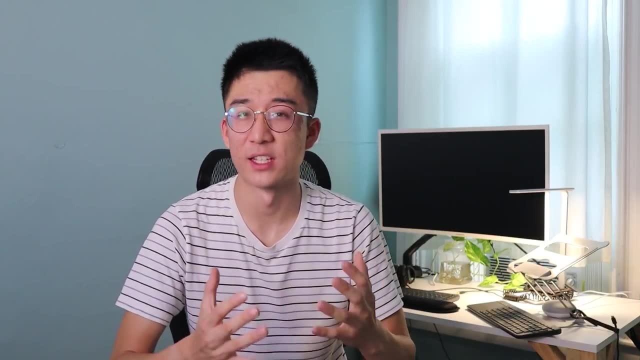 the right method. right, And for someone like me who is decent at engineering, I would have that intuition at times. but there were other times where I could have used some help in developing. But the thing is, if I didn't ask other people for help, then there's no way that I could have gained. 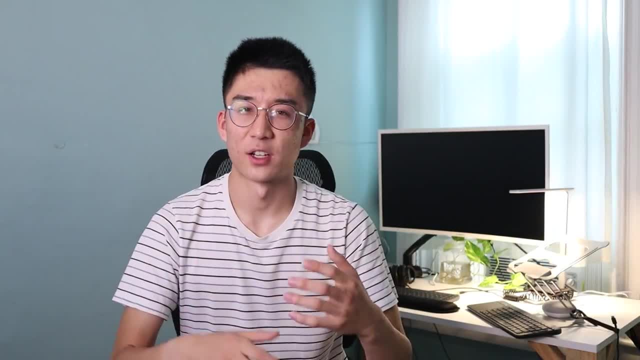 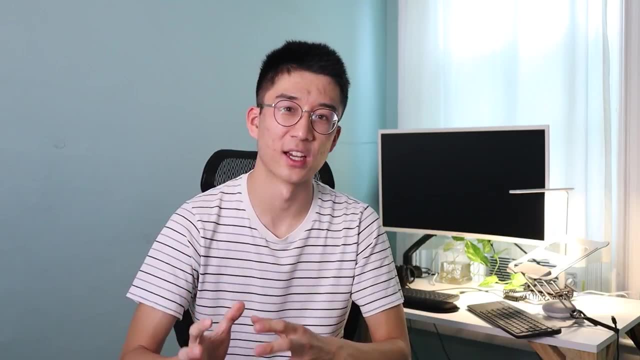 that other perspective and actually learned. So I realize now that's kind of like a strength of working in a team And I think that's one of the things that I've learned over the years is that you can learn from other people and how they approach the problem and then use that insight. 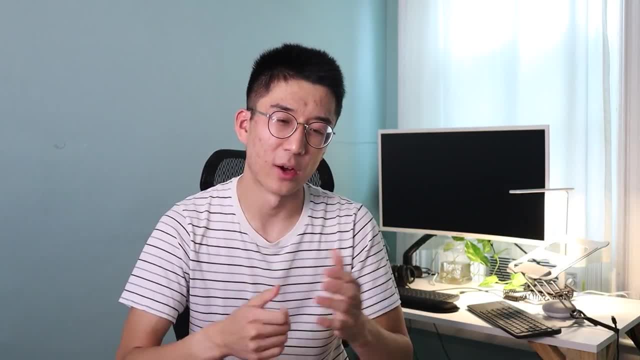 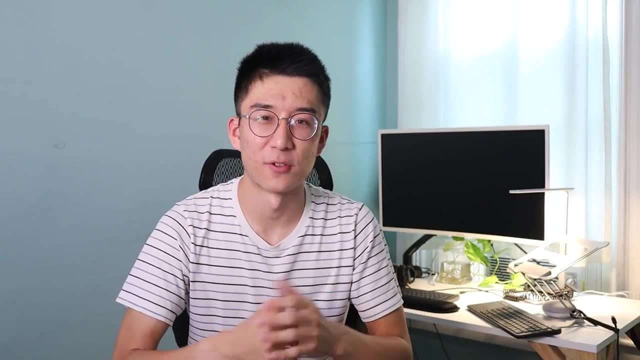 to improve how you yourself solve the problem. So I didn't really realize that as a freshman. I just kind of thought, well, I'm competing with everyone, So you know, I just have to work alone. And I really suffered And I think I wasted a lot of time just by doing that. I knew people who 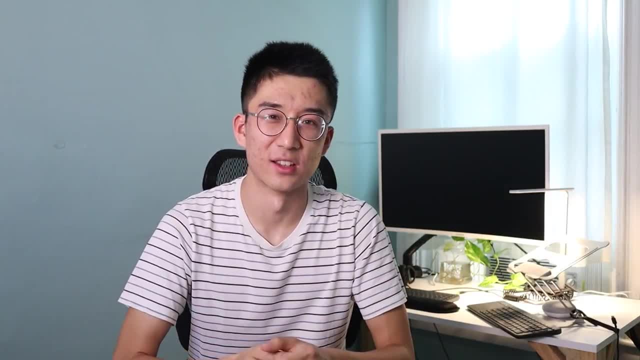 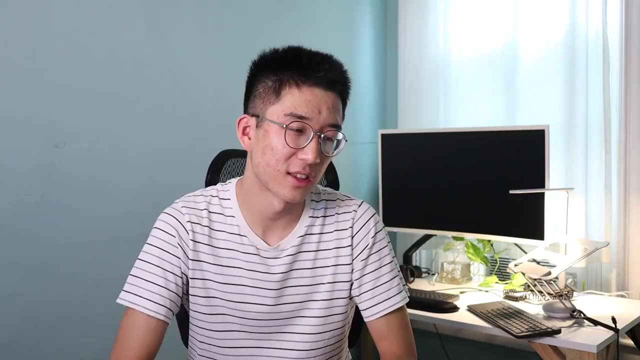 pretty much did their whole problem set at office hours and they would just sit with other students, they would work together and then they would consult the TA or the professor if they needed help And honestly, that would have been a move. I started that freshman year. I could have saved so. 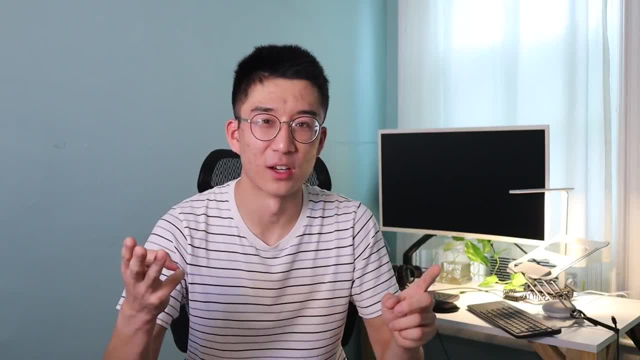 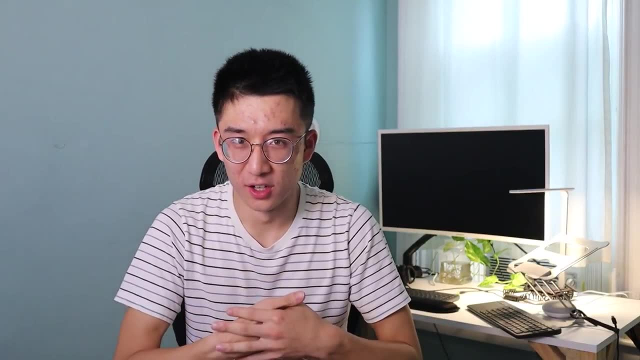 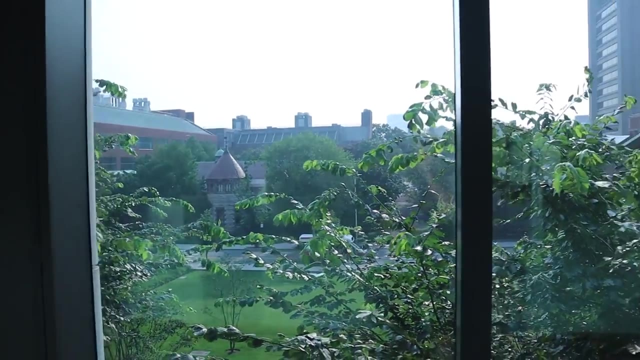 much time, effort and just worry about. you know whether I was going to finish the problem or not, because I was trying to do it myself. I really wish I knew this earlier And, honestly, if you were thinking about going down the same path, don't make that mistake, please, All right. regret number. 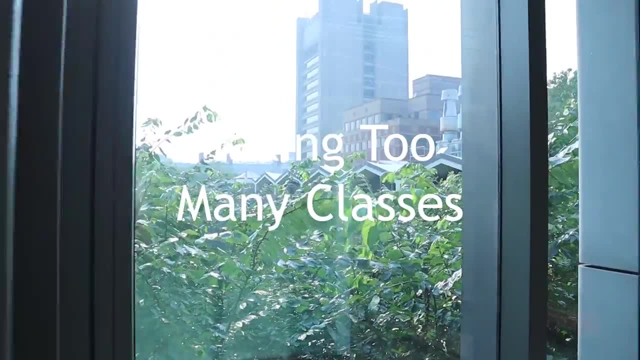 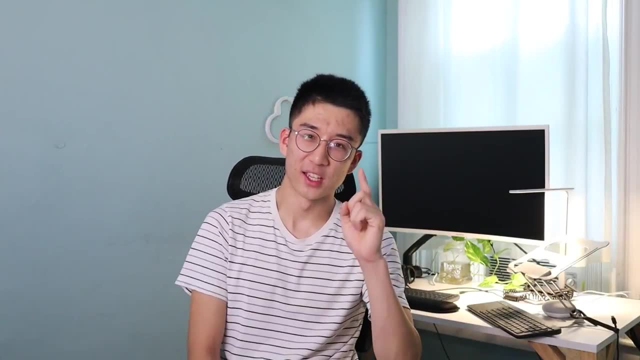 four is taking too many classes. Well, why is that a bad thing, You know? isn't it good to take classes? College is the only time you get to take classes. Well, let me explain why it's a bad idea to take so many. 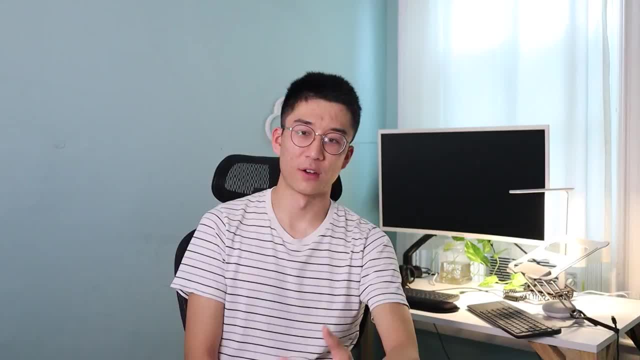 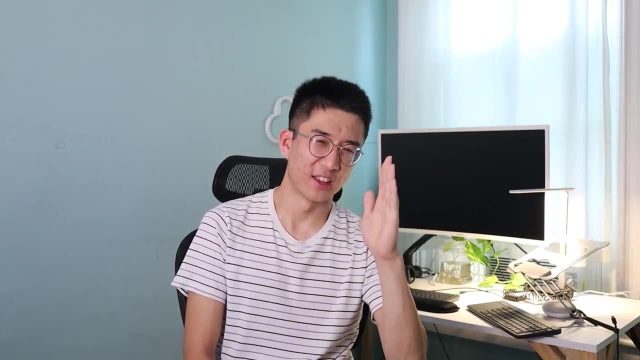 classes. So, coming from a very competitive high school, I was very focused on grades And in college at the very beginning I thought that in order to get ahead, I needed to take the hardest classes and do the best in them, while taking as many as I could. So, because of my previous 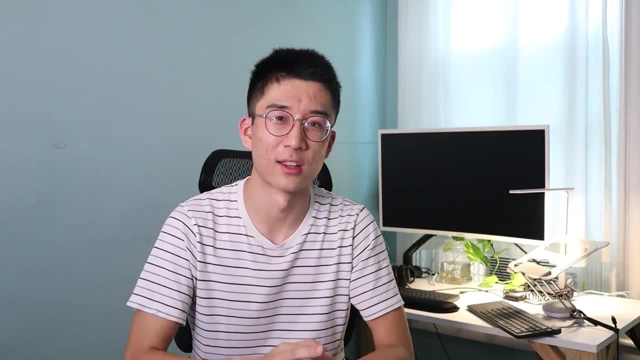 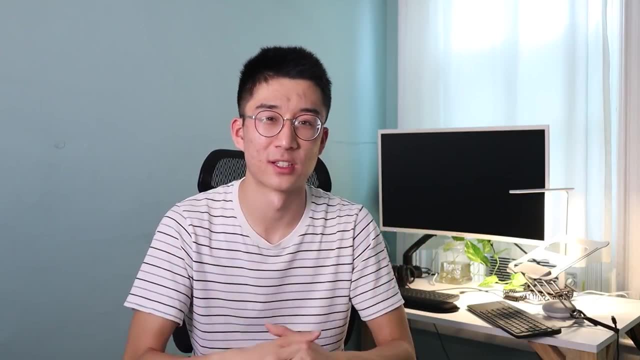 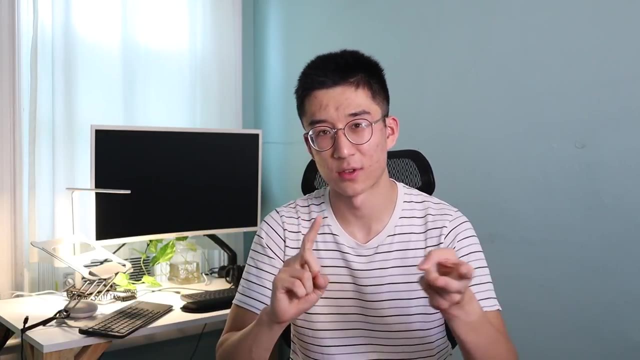 educational background. at that time I was conditioned to think that grades were the sole purpose of my life. I was not even sure what success meant for me at that time. So because of that, I spent the first two years of college taking the hardest classes, trying to take as many as possible, and 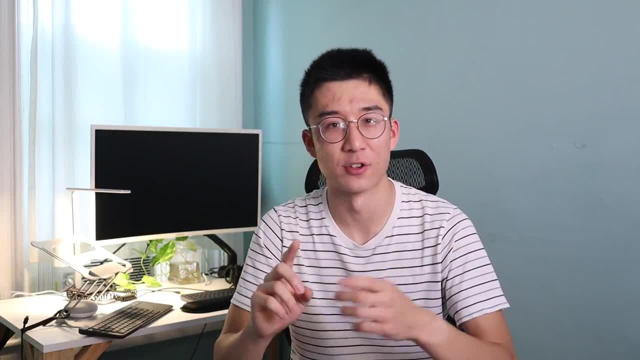 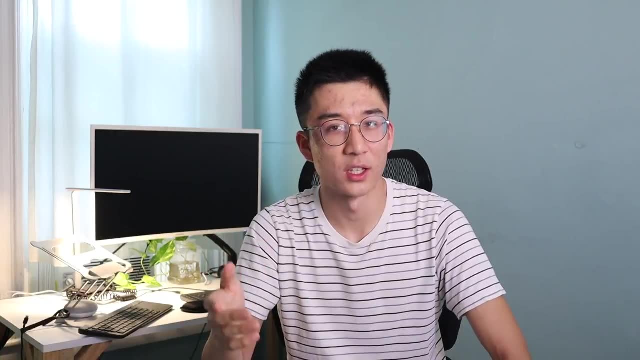 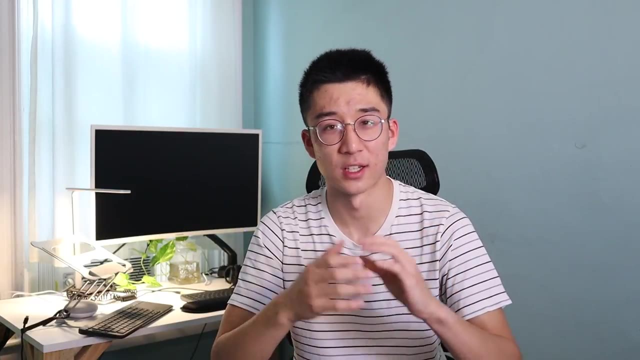 trying to do the best in them And I spent all my time and effort trying to do that. And, looking back, I really wish I spent more time doing research or working in an internship, maybe working for an engineering company or starting this YouTube channel. I feel like things like that outside of. 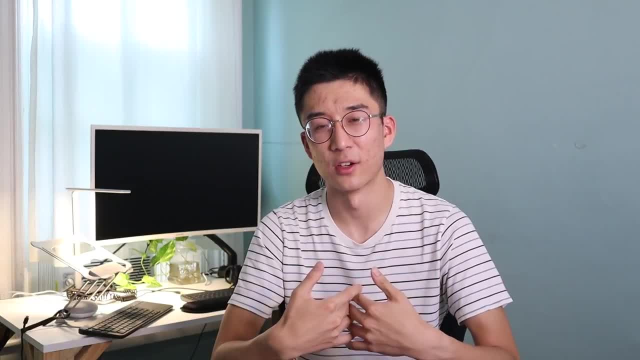 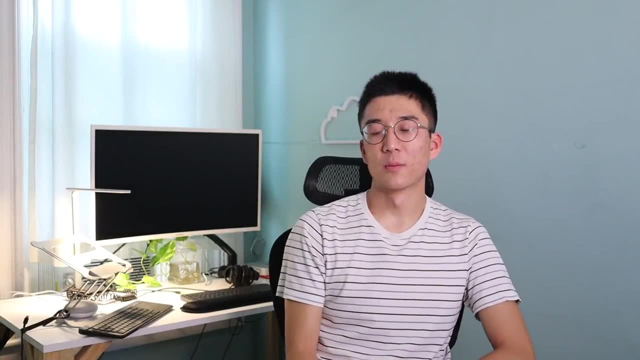 class would have been much more meaningful to me in the long run than, you know, just getting an A in some random class and then forgetting most of the details after the semester ends. Regret number five, my last regret. I probably have many more regrets. I just can't think of them right now because I'm 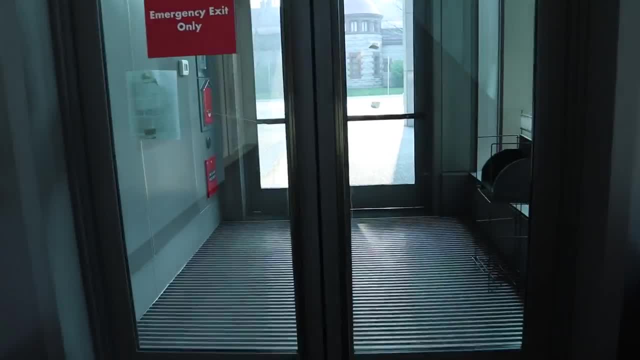 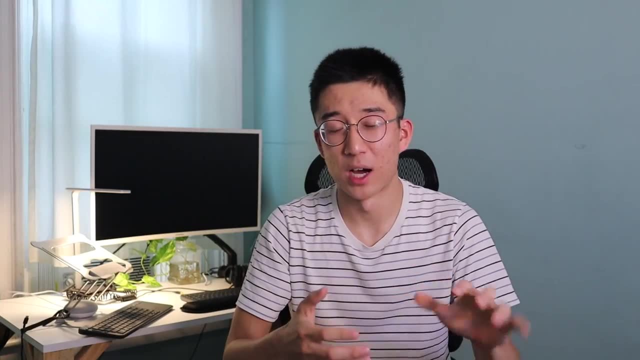 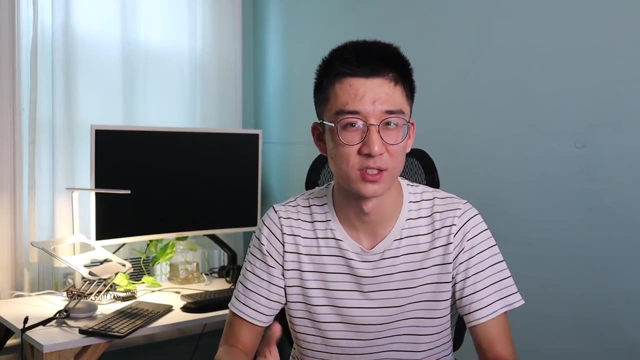 so jaded, you know. But my last regret for this video is that I should have grinded internships earlier. So I think the nature of being a college freshman and starting at the bottom rung of the hierarchy again is that your first few years are kind of just for gaining experience. So typically in the first two years or 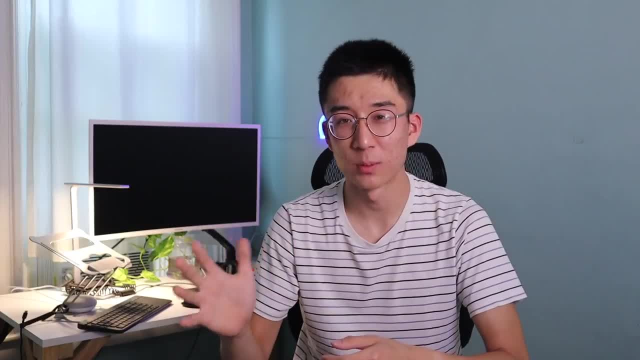 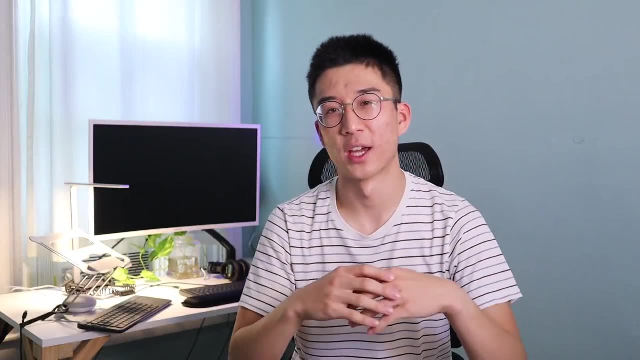 so you're just kind of doing what you can get. It might not be exactly what you want to be doing, but you're doing it just for experience, because that's all you have right now And then eventually, as you gain more experience, you can start to have more of a choice in what you want to do, because 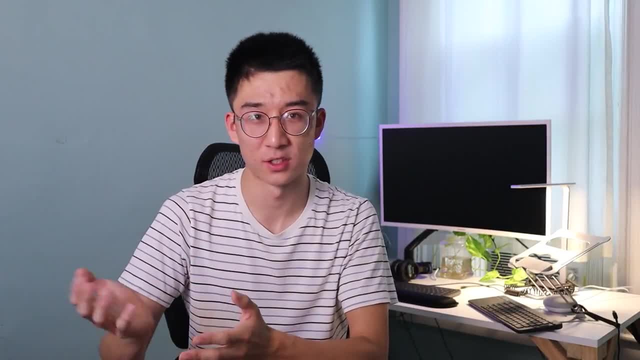 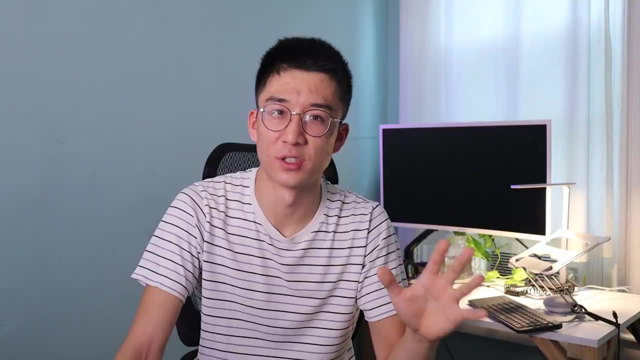 people are going to be looking for those with your skills. The thing is, if you start the whole process earlier, that means you have an edge and you might not have to spend those initial years just doing whatever comes your way. so for me personally, i wish i had looked into. 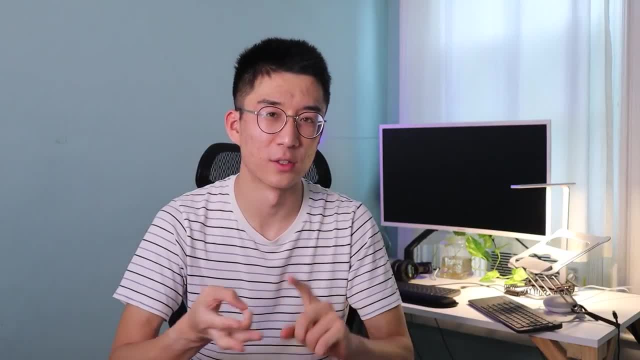 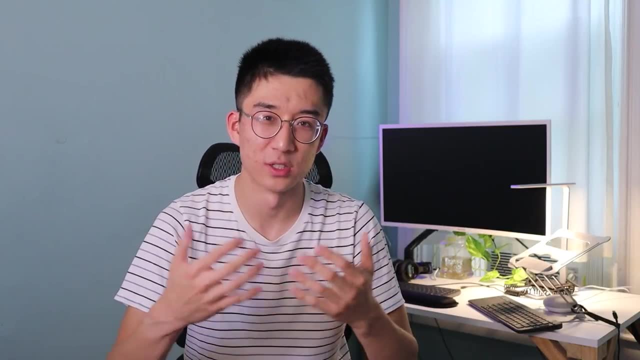 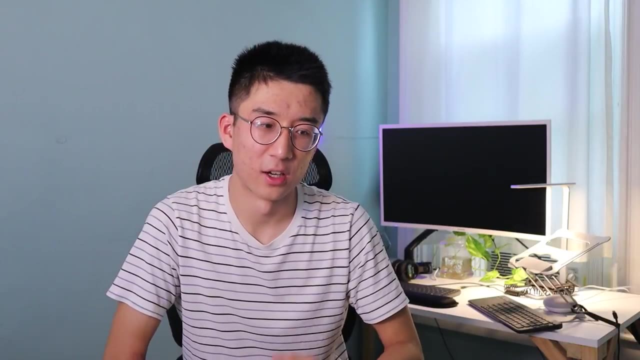 industry internships earlier, network and really developed my job application in order to get those internships, because this summer was my junior summer and i actually was unable to get anything related to biomedical engineering, so i think if i started earlier, my chances would have been better and, honestly, i think this is just about being a go-getter, not being caught up in the miniscule.